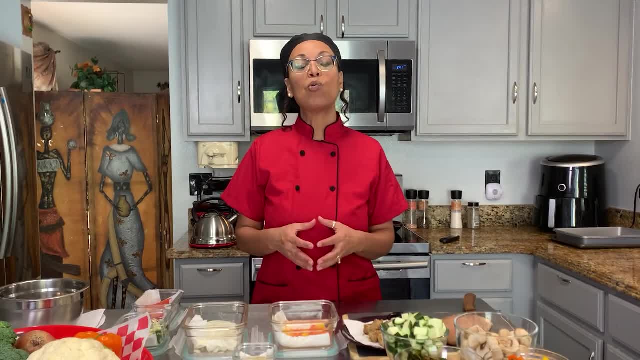 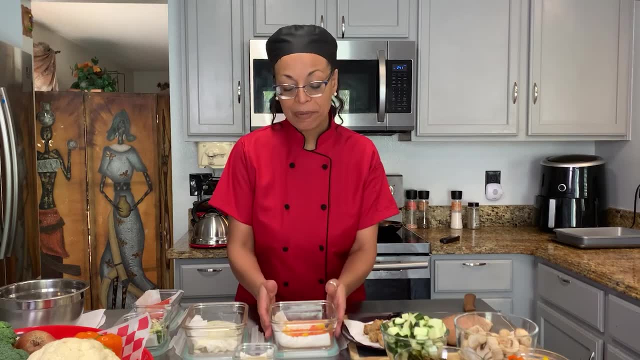 them to be lazy Number three: there's a lot of wives who need a lot of garden tools and they good to have some mundane home-cooked food. One of the things I love about cooking in the kitchen is that when we want to be with your kids, we have the way. thatpartPs. 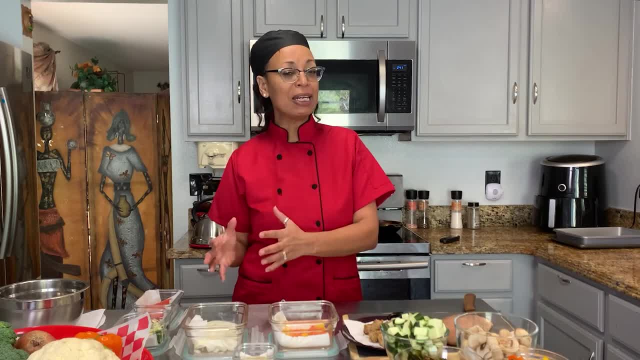 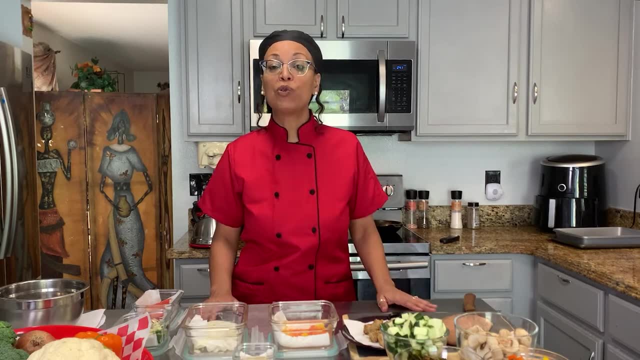 that they have many. If we were to cook every single meal in our living room, eating meals even if di or so much, and find recipes where you could combine them so they could enjoy the nutrition at the same time as they enjoy flavor. 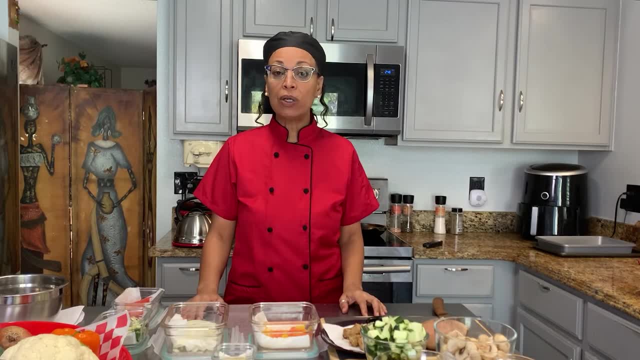 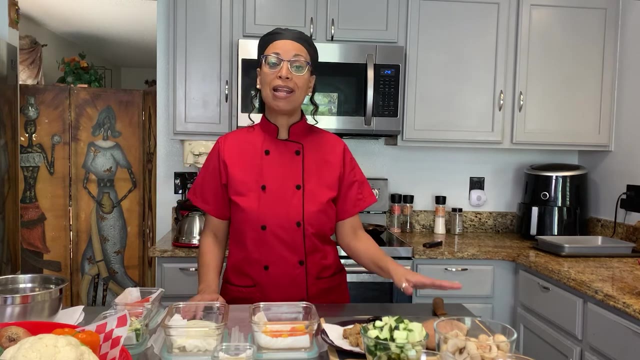 Number four: safety. first, Make sure that kids understand when they come in the kitchen that although this is a fun place to cook, safety is important. that they understand that the kitchen has a stove that is hot and they cook it burnt, that knives are sharp. 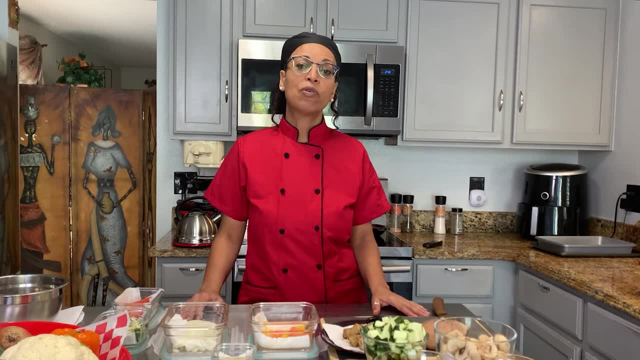 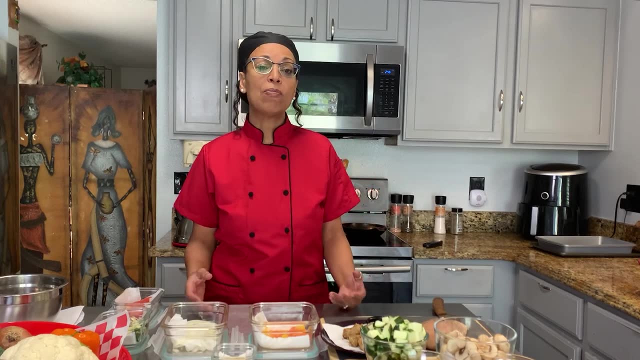 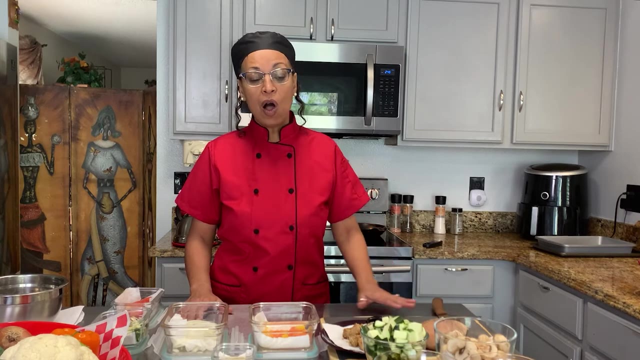 and also consider using alternative tools. For example, instead of using a sharp knife, you could have the kids use some type of equipment that could make vegetable chopping easier without the need for a knife blade. Also, they can rinse the ingredients, the food. 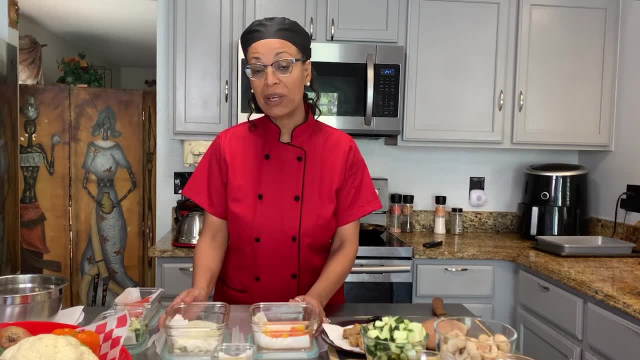 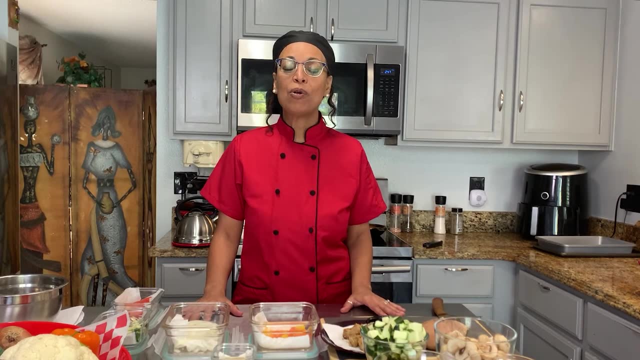 they could label it. There are so many things that you could get the kids involved, and the competitive advantage that they will gain by learning how to cook safely will be with them for the rest of their lives. So thank you for joining us for this meal prepping video. 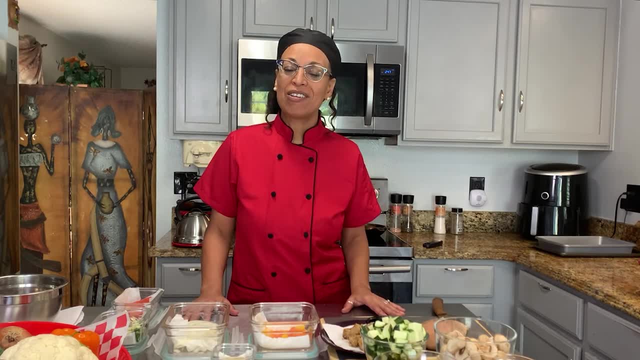 and we hope that you continue to enjoy the content that Orange County Library System is releasing for you. For more information, go to oclsinfo and find out more about videos, books, resources and community events at the local library. Click on the description below for steps. 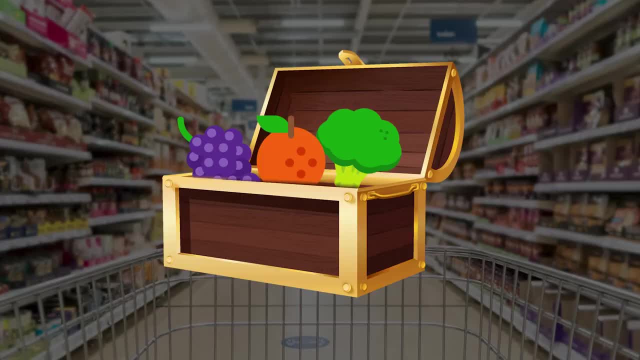 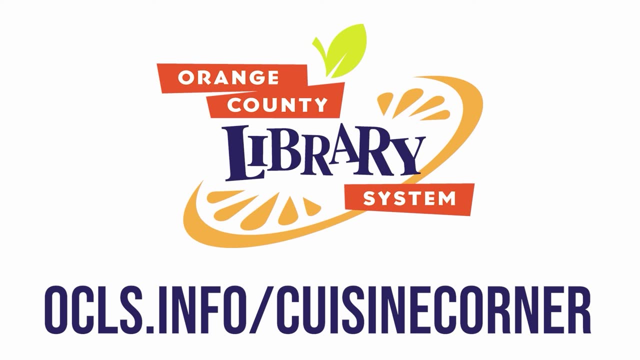 on how to get the kids involved with a grocery store treasure hunt. Thank you for watching. To learn more about Cuisine Corner and see more videos, visit oclsinfo. slash cuisine corner. Orange County Library System is your place to learn, grow, connect.